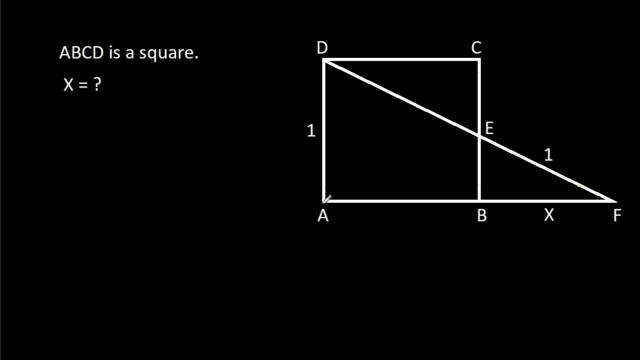 In this video we have been given that ABCD is a square and AD is a 1,, EF is a 1, and BF is X. Then we have to find X. So we know that ABCD it is a square. That means AB it. 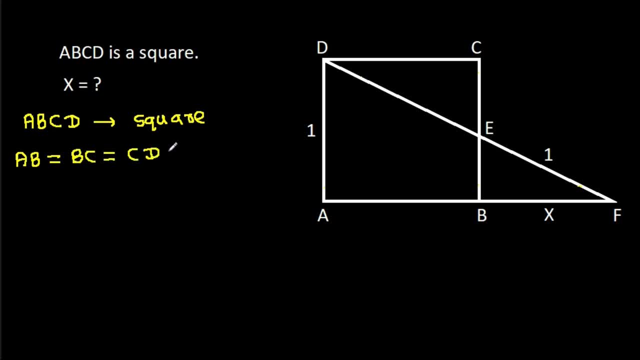 will be equal to BC, it will be equal to CD and it will be equal to DA. That is 1.. So AB is a 1,, CD is a 1, and also these angles, they will be 90 degree, And AB it will be. 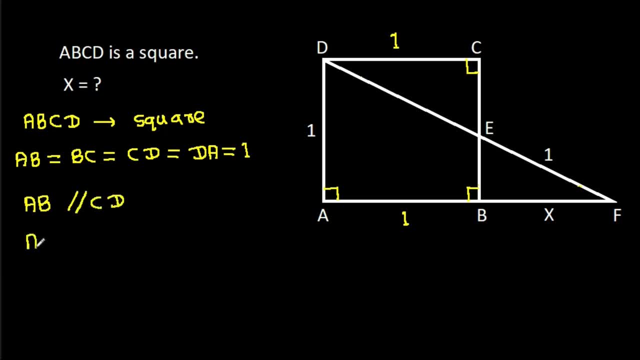 parallel to CD, So AF it will be parallel to CD, So angle AFD it will be equal to angle CDE. Suppose theta These two angles, they will be equal. suppose theta And and and and. 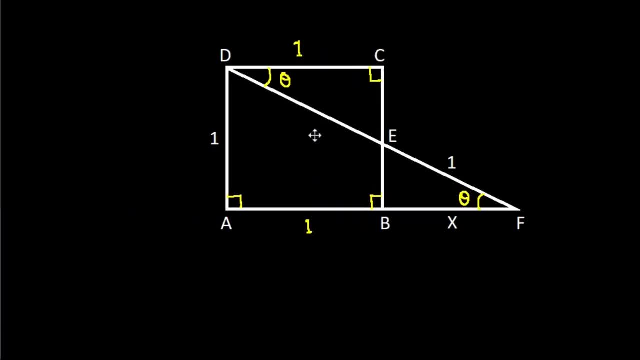 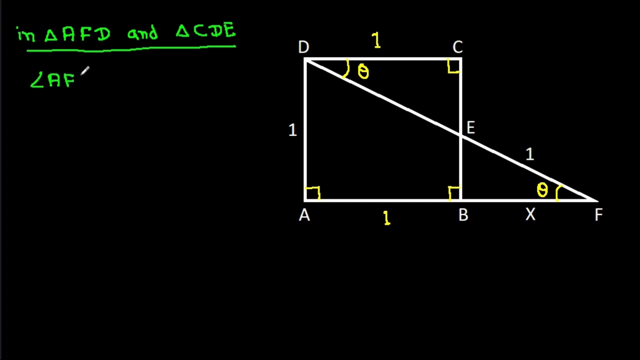 and, and and. Now in triangle AFD and triangle CDE we have angle AFD is equal to angle CDE, that is theta, and angle DAF is equal to angle ECD, that is 90 degree. 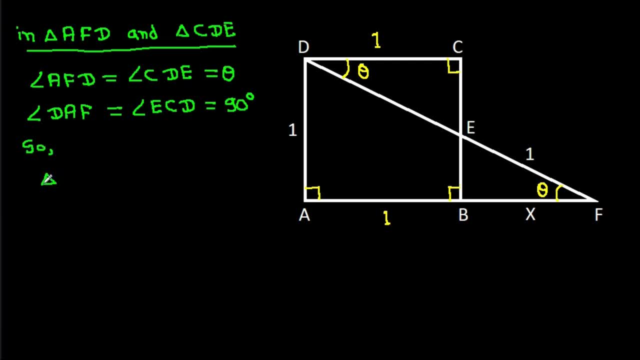 So triangle AFD. it will be similar to triangle CDE, Hence AF over CD, it will be equal to AD over CE and AF it will be 1, plus X. it is 1, plus X over CD. 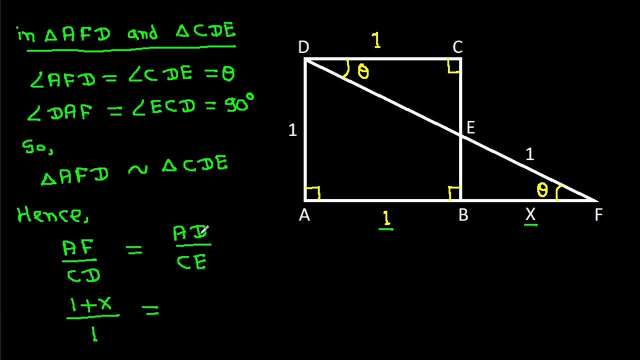 It is 1, plus X over CD. It is 1, plus X over CD. It is 1, it is equal to AD is 1, over, and we know that BC it is 1.. So if CE is A, then BE it will be 1 minus A. 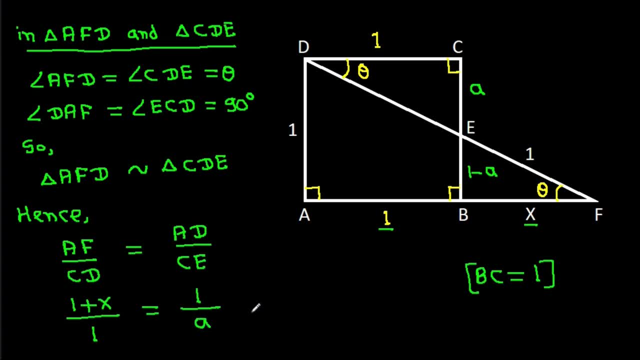 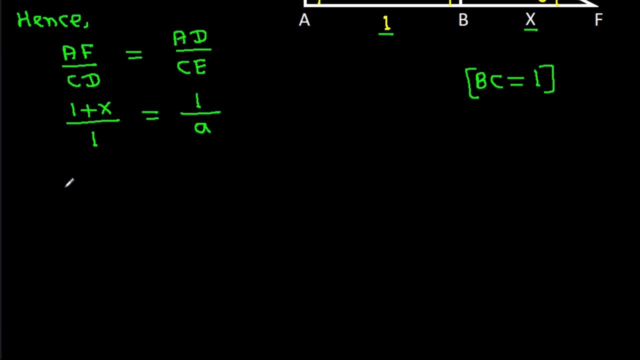 So CE it is A, And if we cross multiply then A times 1 plus X it will be 1 times 1, and it is A plus AX is equal to 1.. So A, it is 1 minus AX. 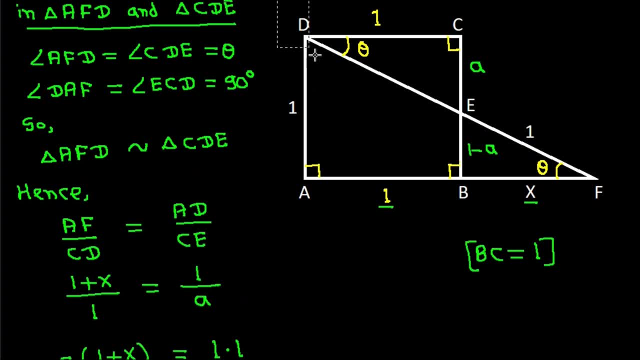 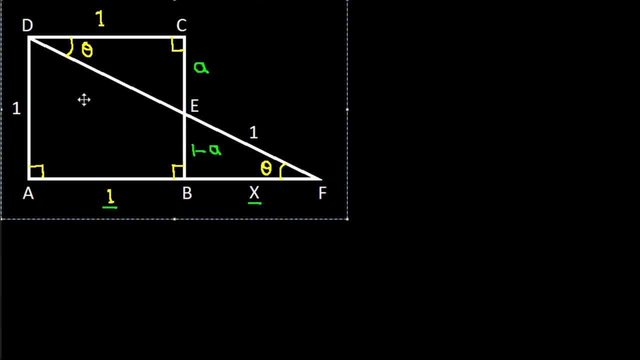 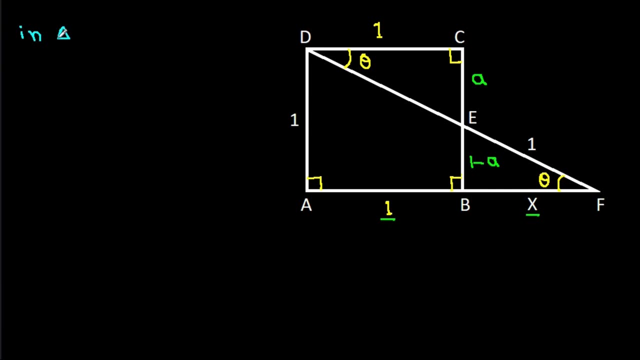 And now, if insanek is equal to 1, it goes. B, then wider angle: overragen is equal to 1, overreme it is wider angle over refere at 15, and B it will be 2, over 14.. 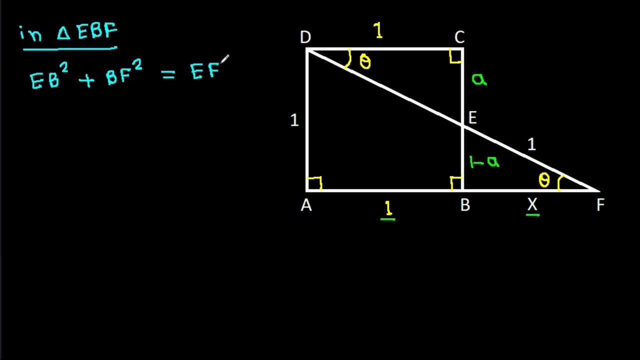 And These two areие plots. And if a is equal to is equal to, a is equal to b, EF square by Pythagoras theorem, because this angle, it will be 90 degree, and EB is 1 minus A square, plus BF is X square, it is equal to, EF is 1 square and it will be 1. 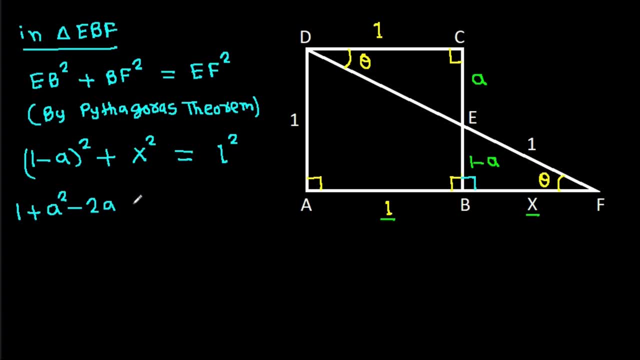 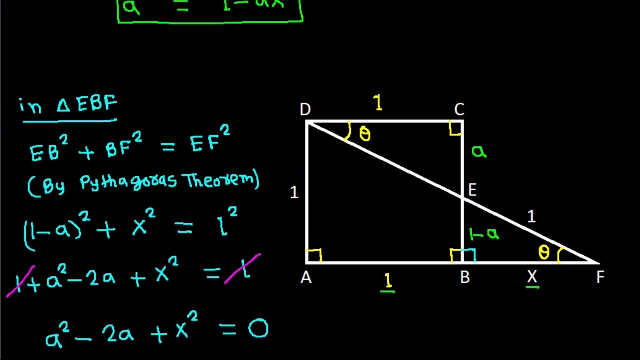 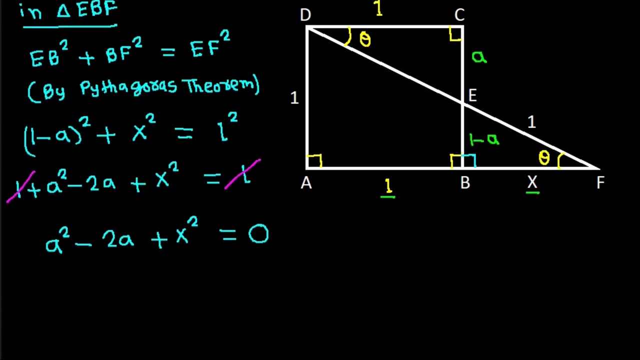 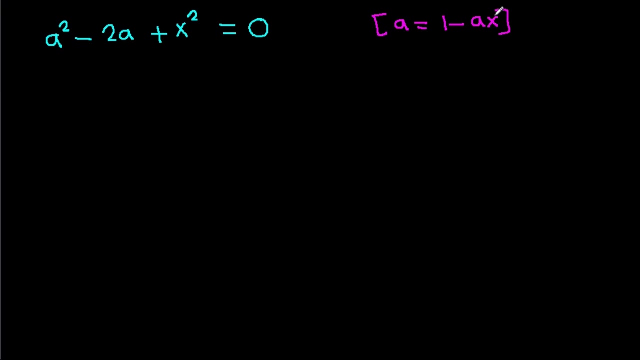 plus A square minus 2A plus X square is equal to 1 and 1 will get cancelled. So A square minus 2A plus X square, it is 0 and we have A is 1 minus AX. We have A, it is 1 minus AX. 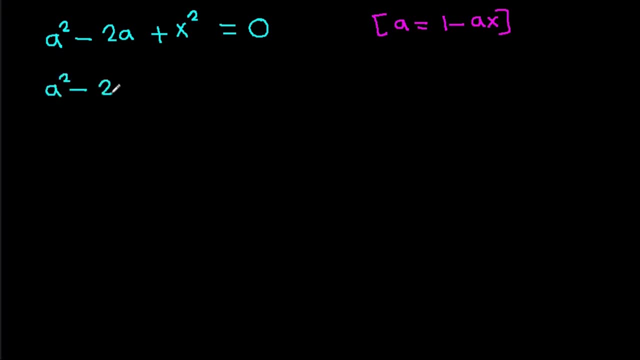 So it is A square minus 2 times A is 1 minus AX plus X square- it is 0. and it is A square minus 2 plus 2AX plus X square: it is 0.. So A square minus 2AX plus X square: it will be equal to 2.. 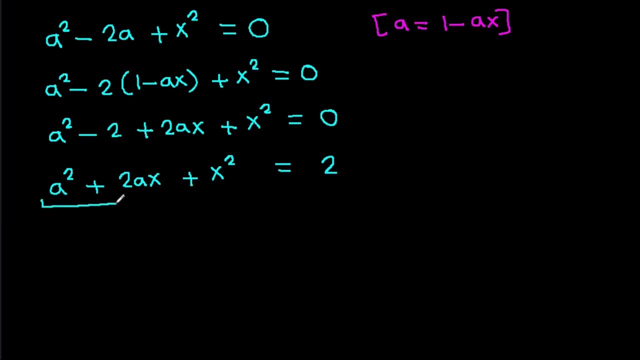 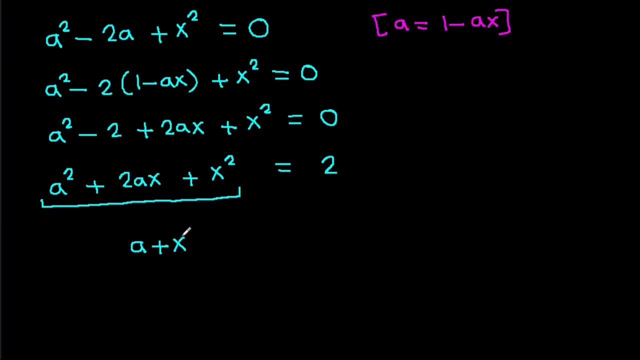 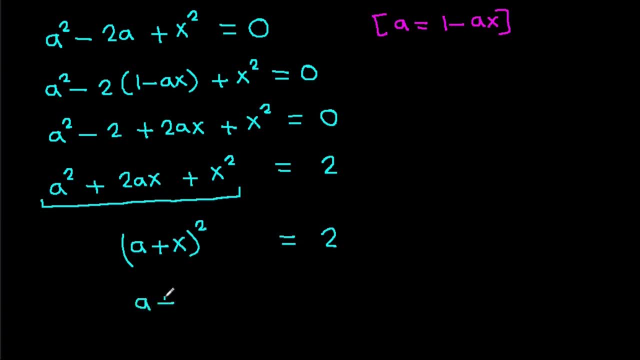 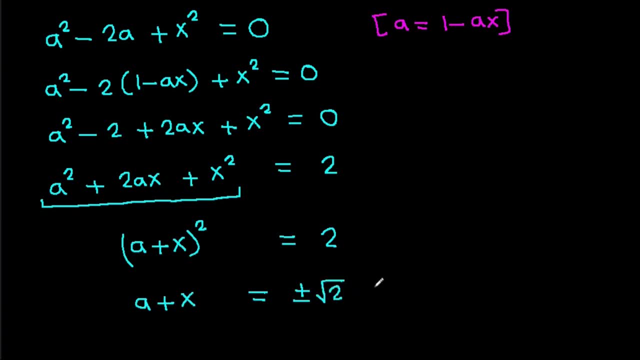 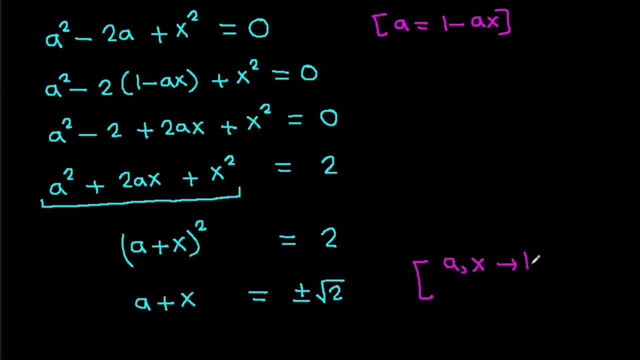 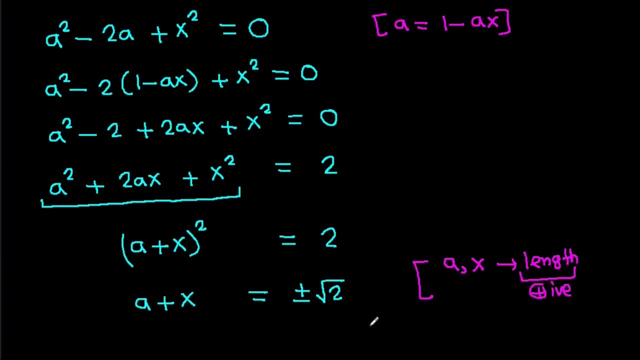 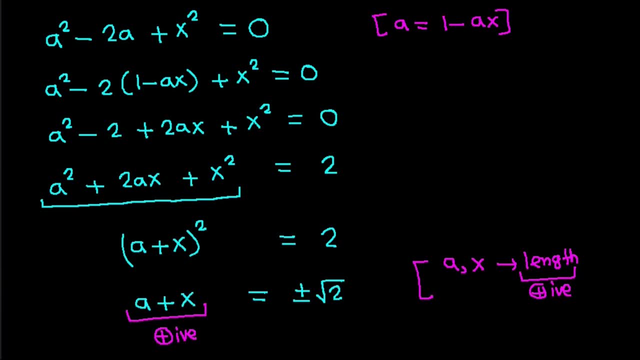 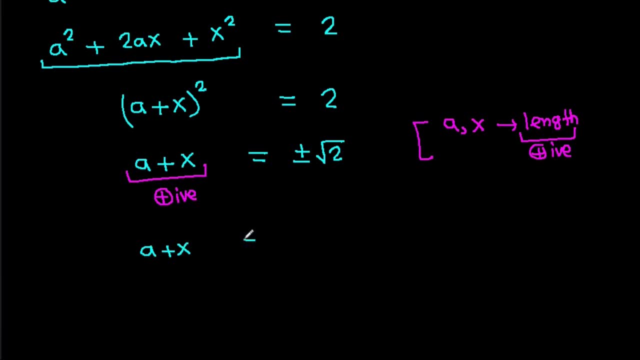 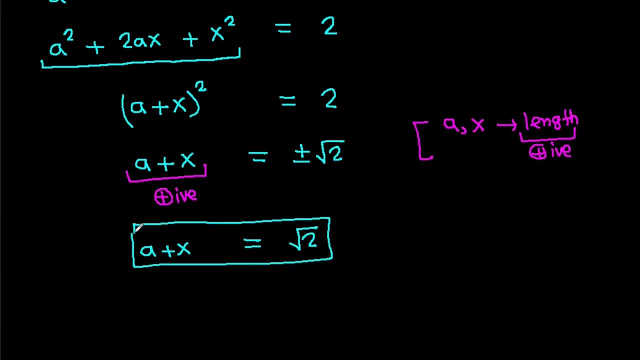 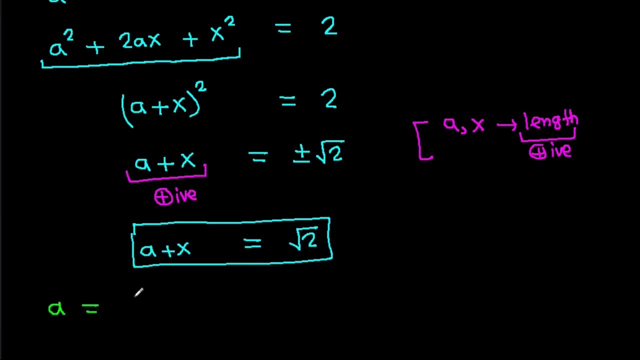 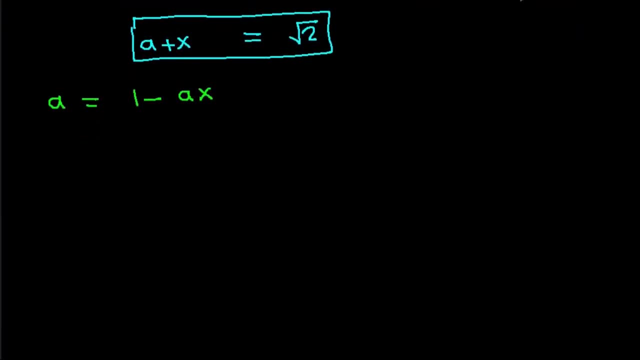 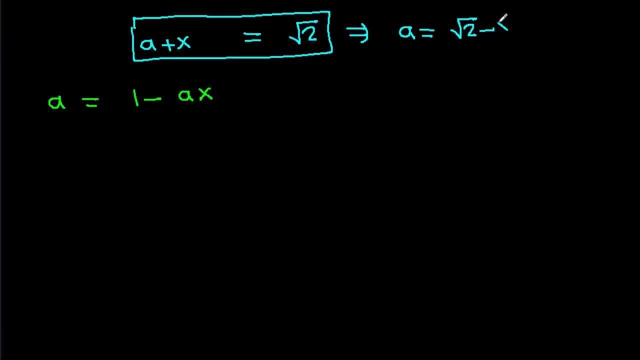 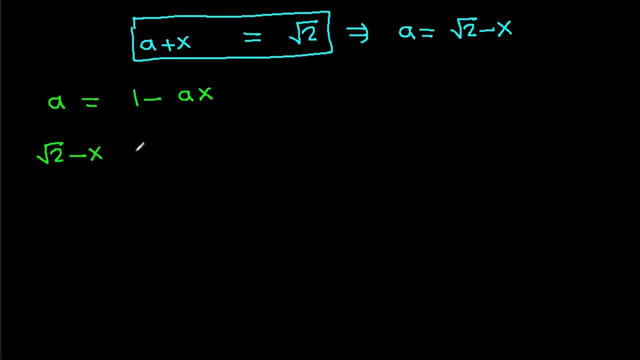 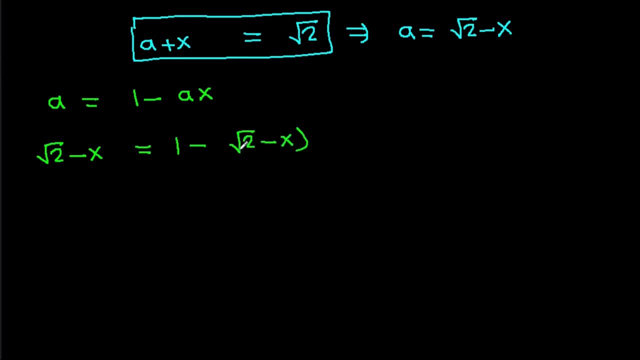 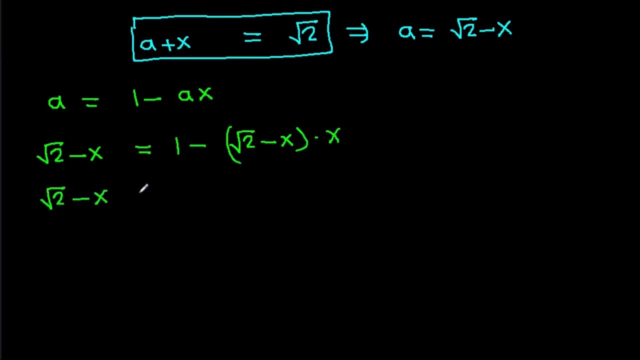 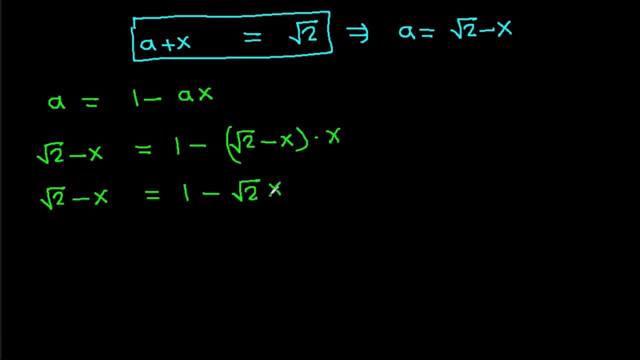 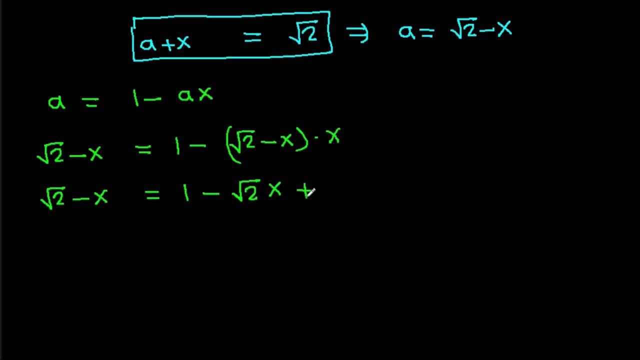 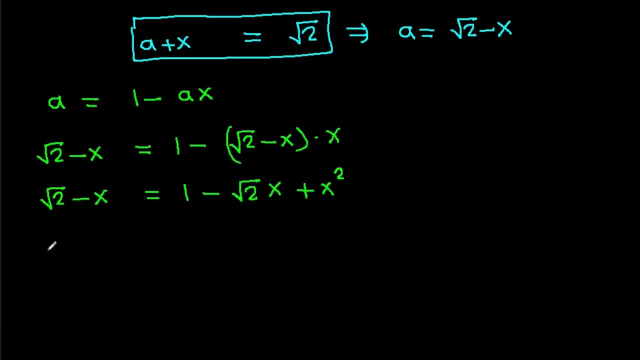 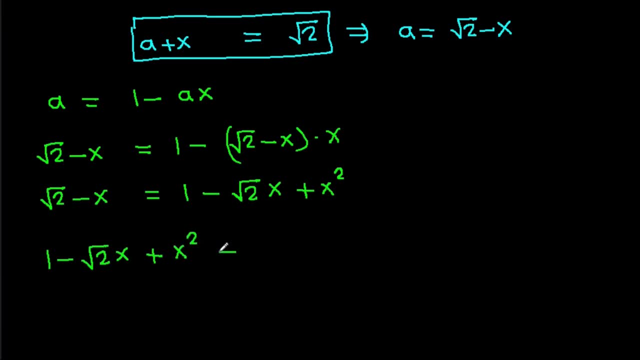 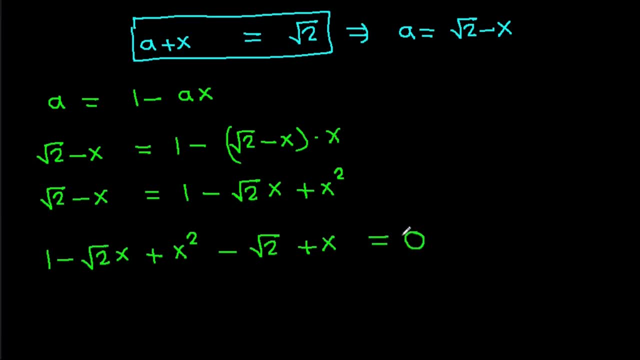 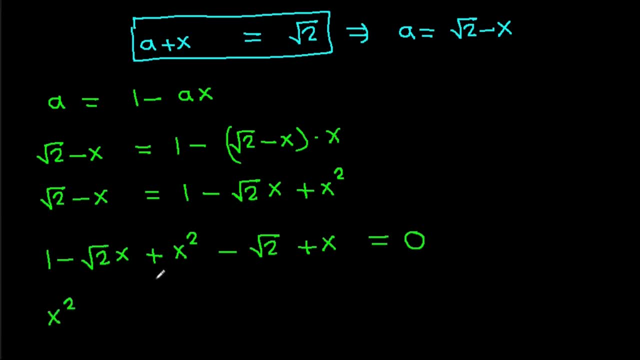 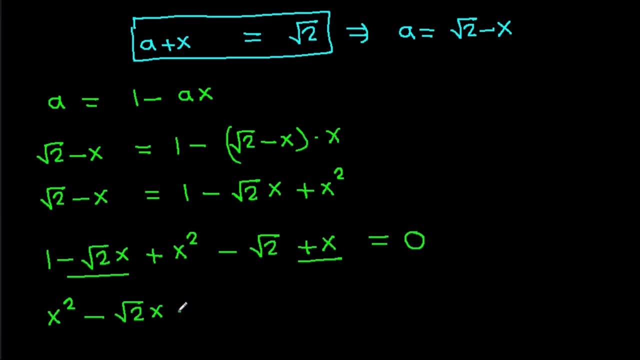 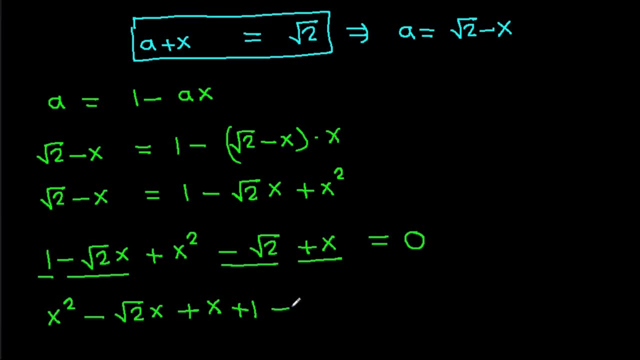 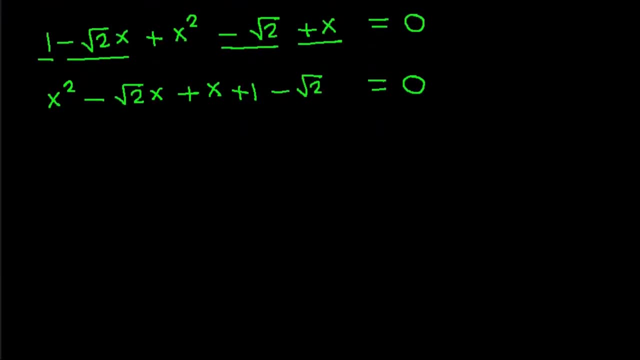 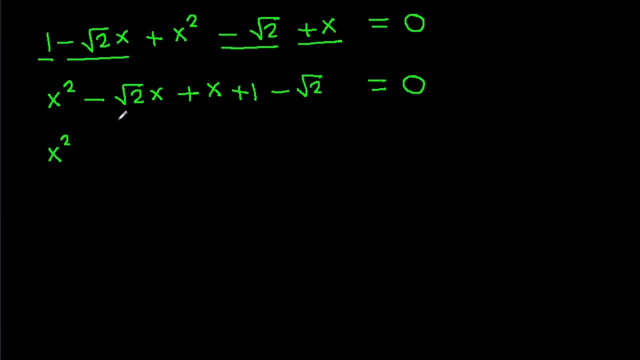 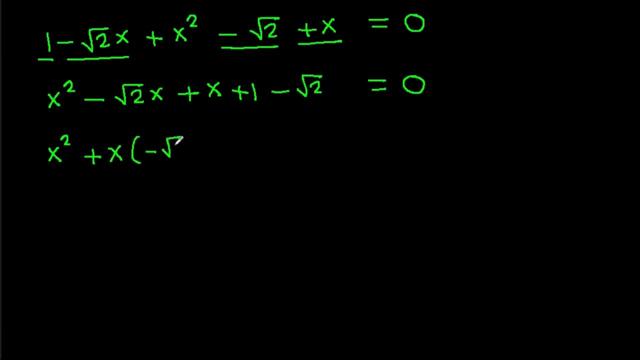 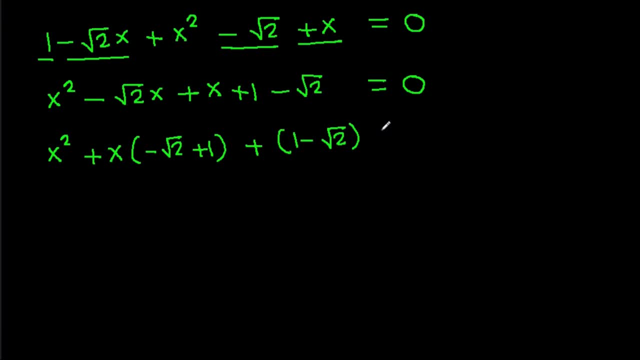 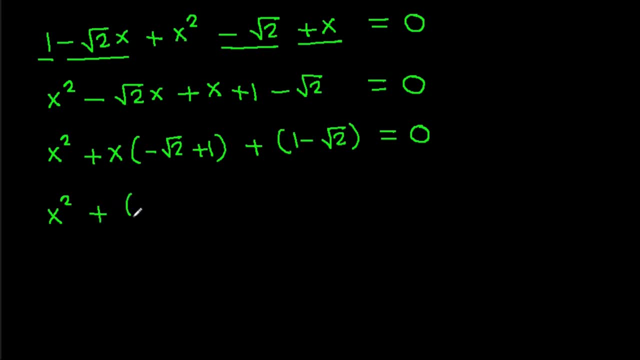 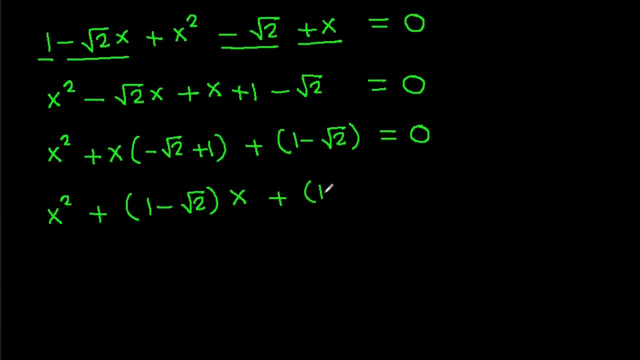 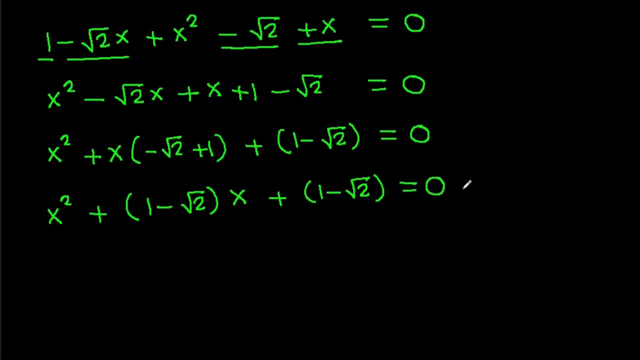 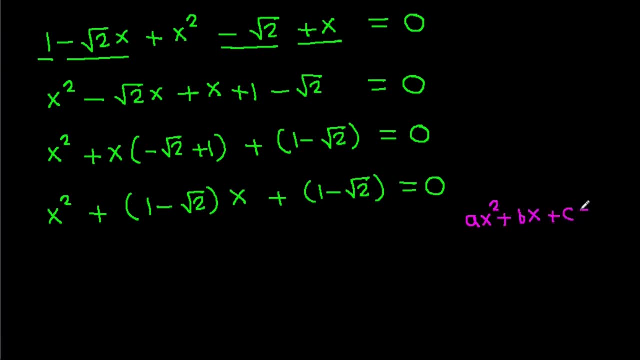 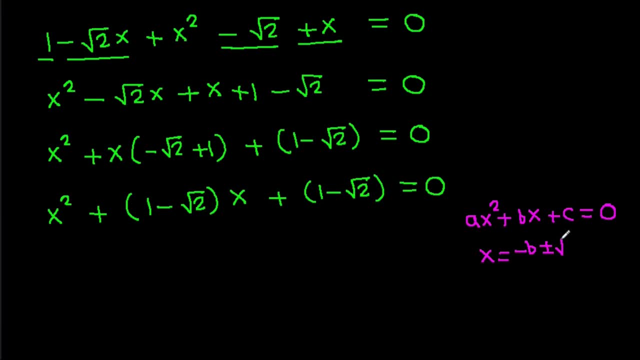 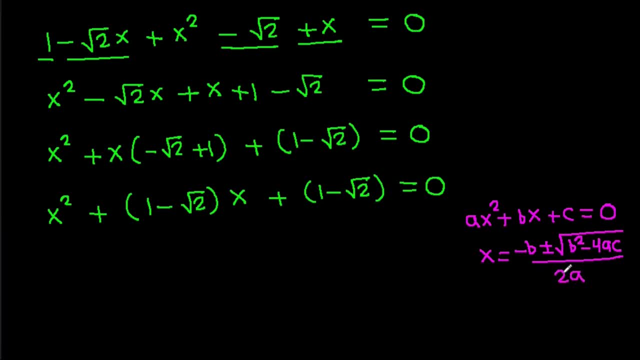 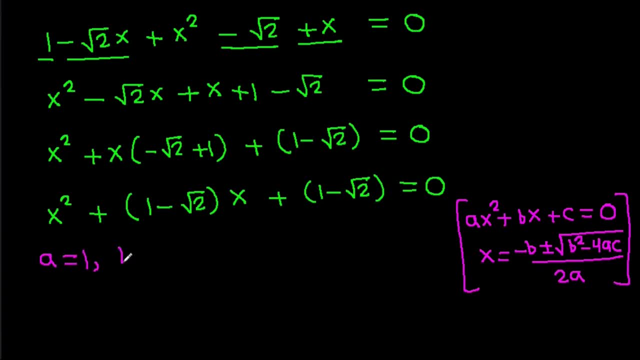 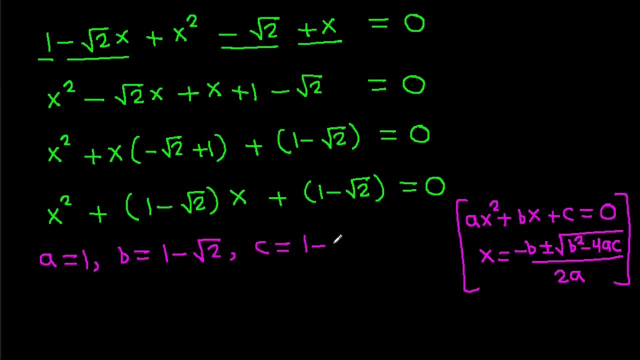 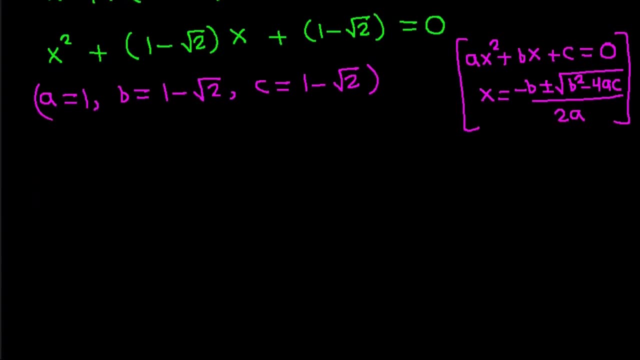 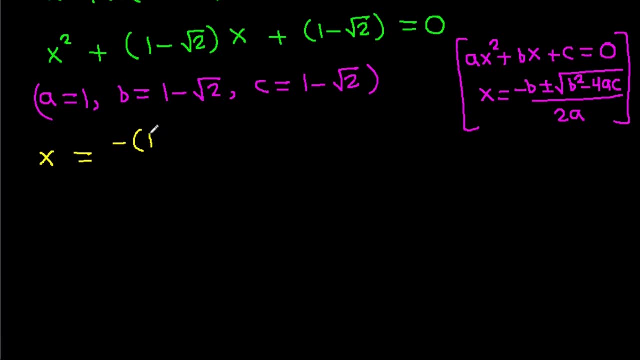 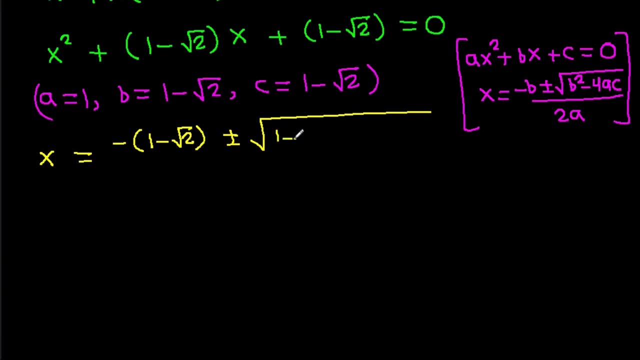 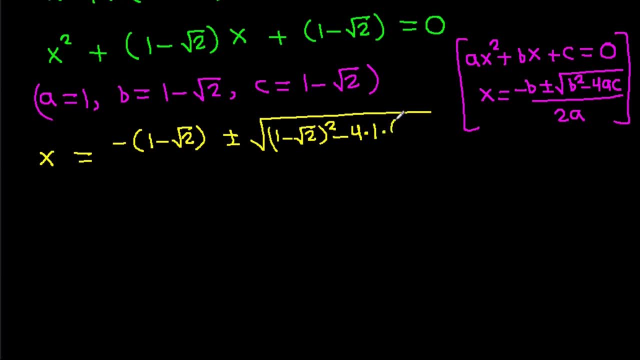 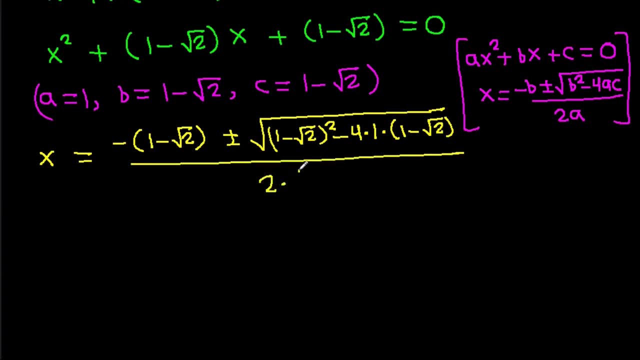 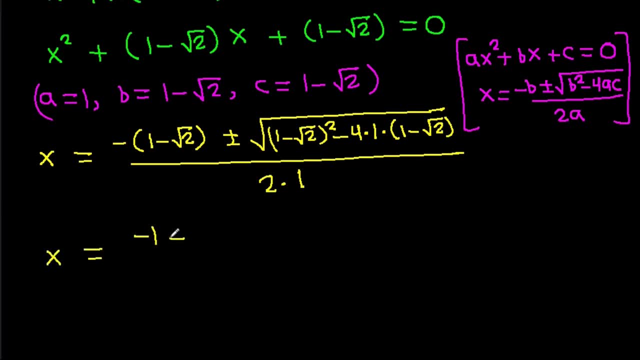 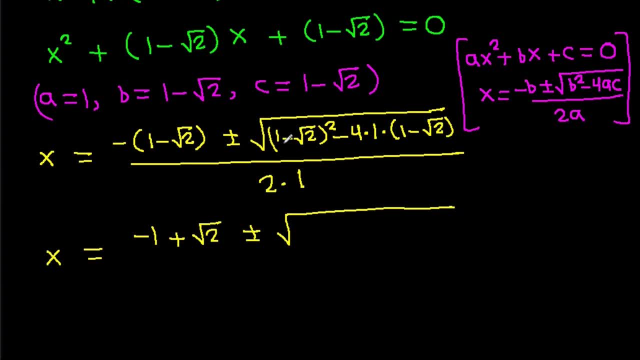 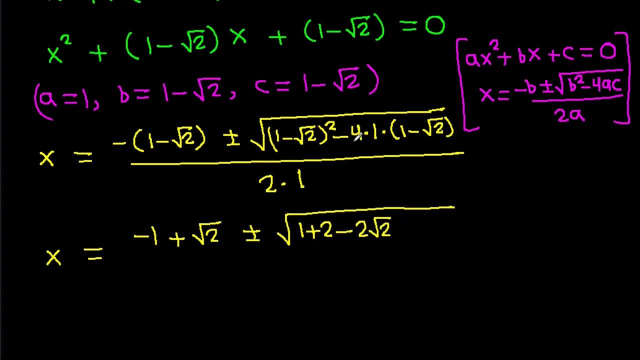 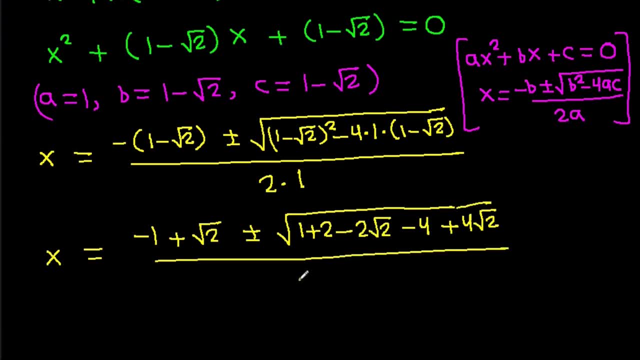 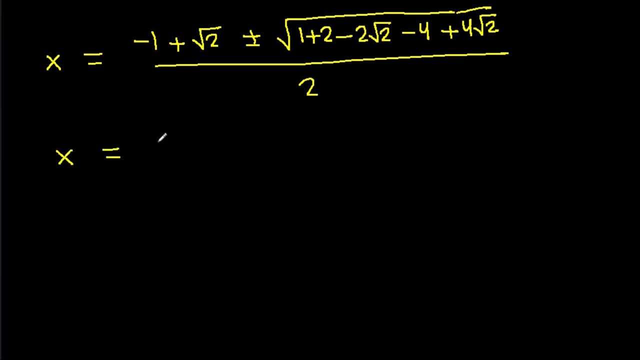 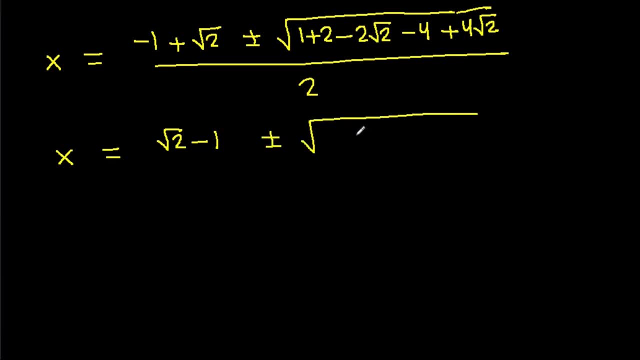 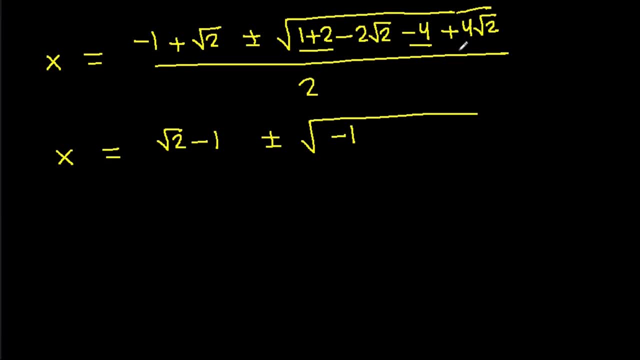 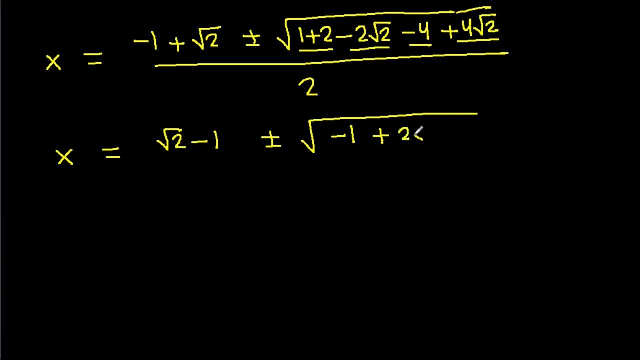 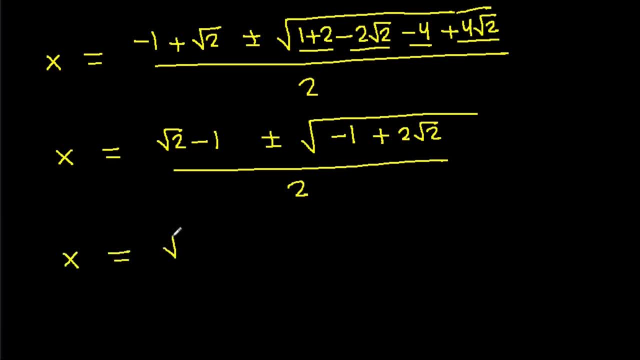 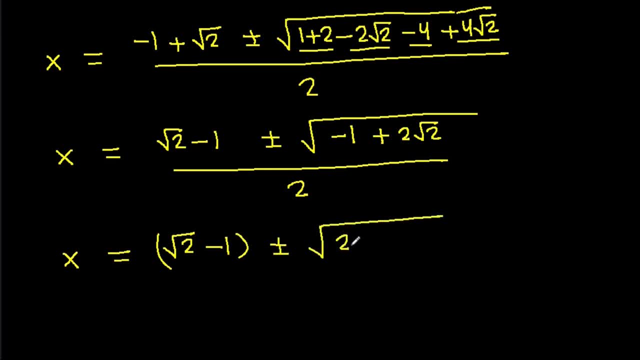 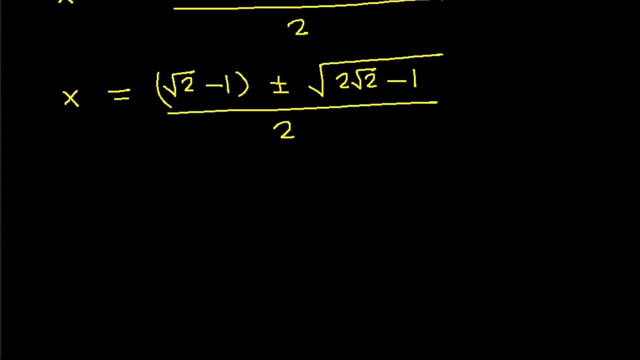 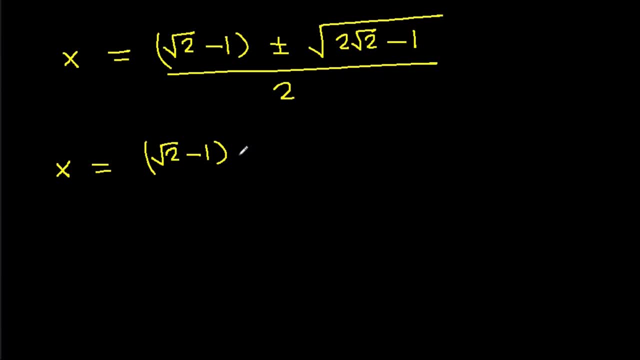 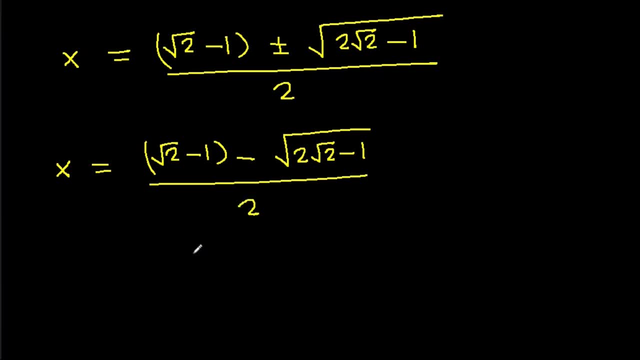 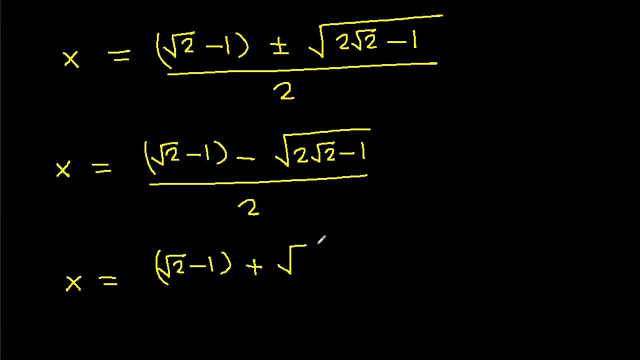 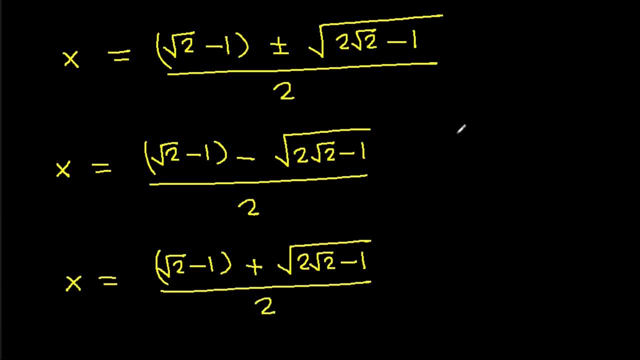 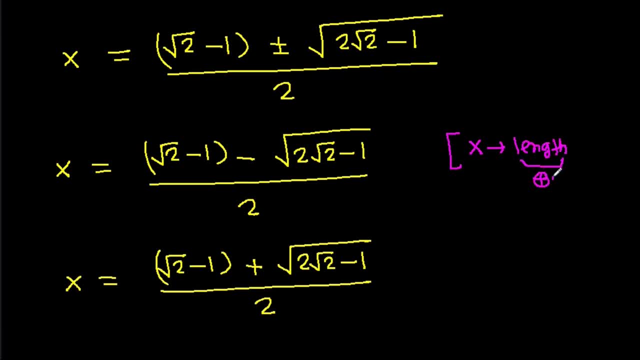 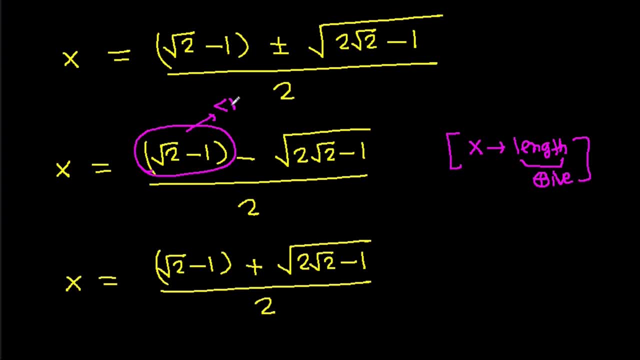 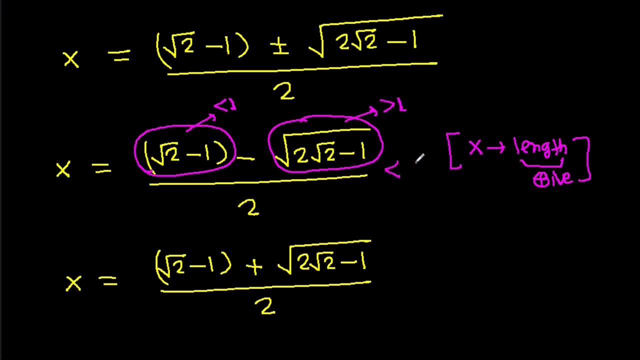